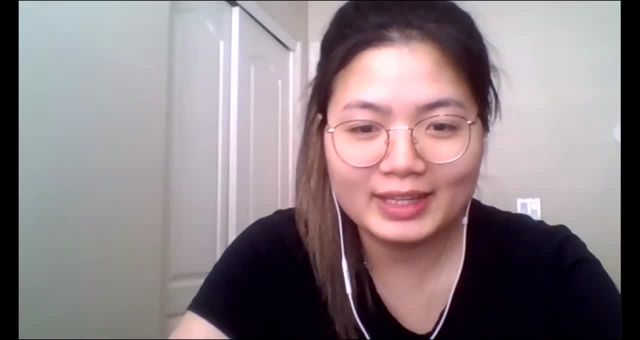 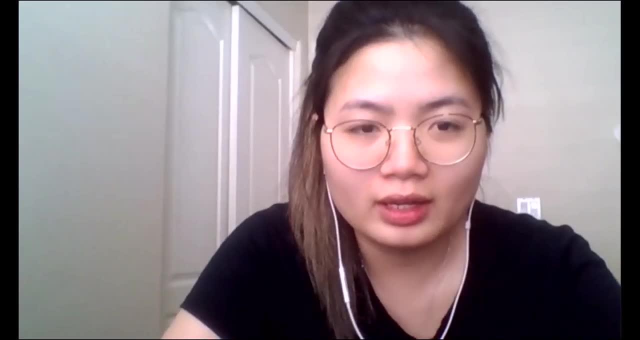 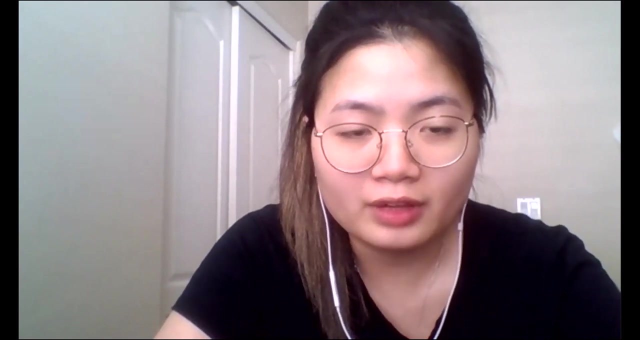 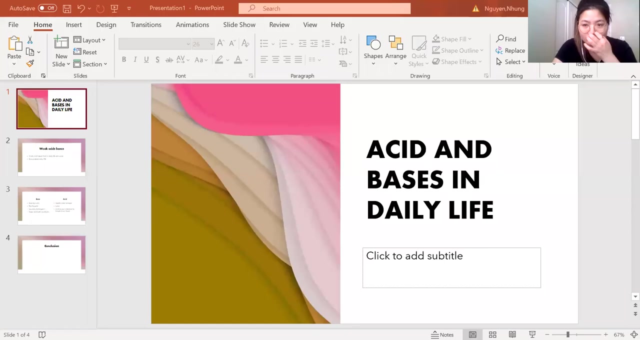 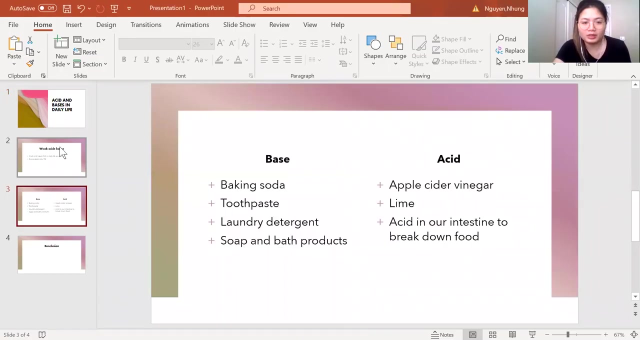 Hello, this is me. Now I'm doing the presentation about ACID and BASIS. And I'm using Zoom, because this has a feature that I can share my screen, so I can share the slide PowerPoint to do my presentation. And so this is my slide PowerPoint. And it's only a draft, so I don't have much here. And I will put some more pictures here to make it more colorful. But this is basically how I do my presentation. And there's still the face on the right corner, the upper right corner. So you can still see me and you can still see my slide PowerPoint. And I'm using Zoom, because this has a feature that I can share my screen. 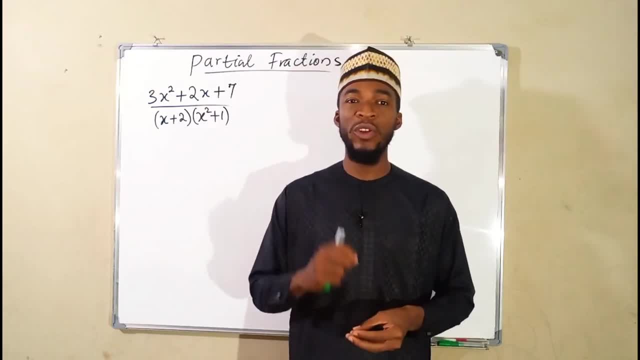 Hello, good morning viewers. Still on to how to dissolve profile compound fractions into partial fractions. I have another problem here which falls under the first category. 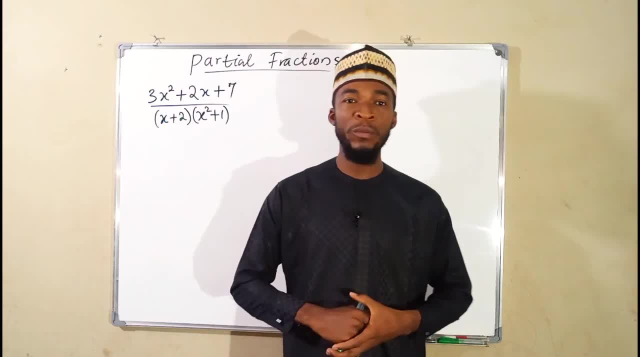 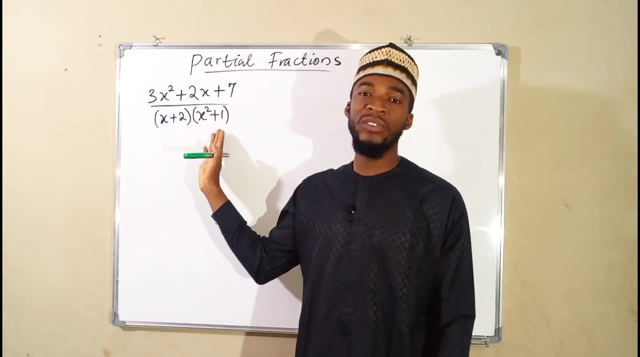 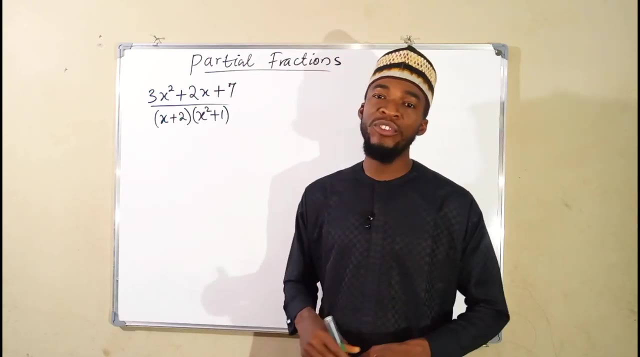 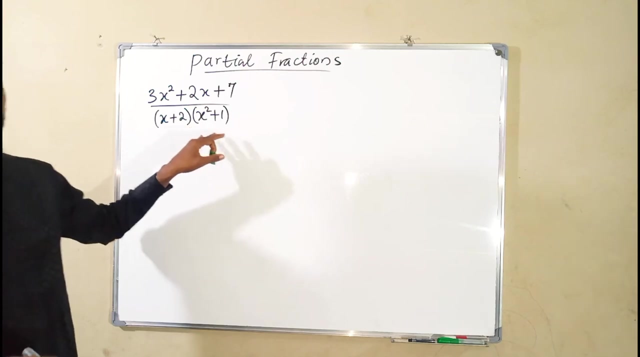 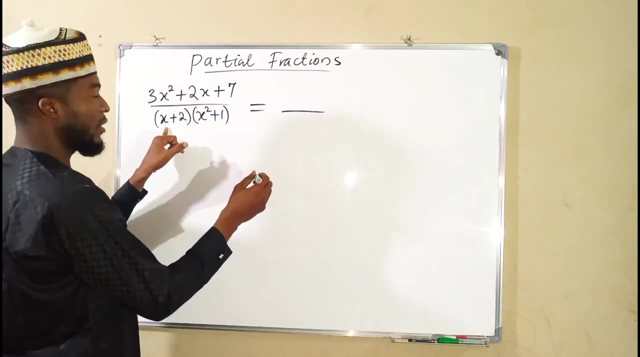 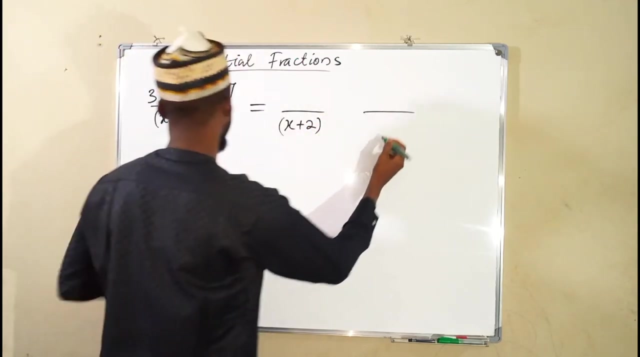 You can see we have two different factors under the denominator. One is linear factor and the other one is quadratic factor. Suppose this quadratic factor can be factorized, we have to factorize it in order to obtain three separate factors. But since it cannot be factorized, let me show you how to dissolve this into partial fractions. You know because we have two factors, we are going to obtain two separate fractions. So the first one will contain this factor as its denominator, x plus 2. And the other fraction is going to contain the other factor as its denominator.